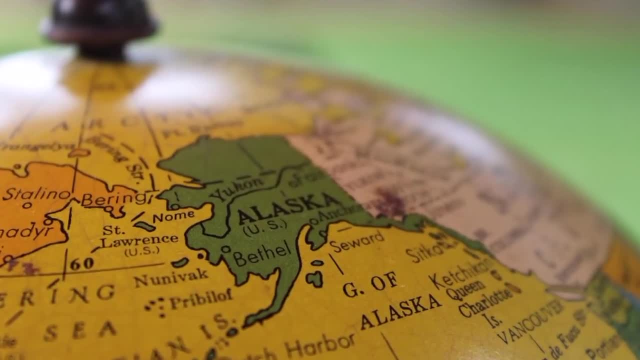 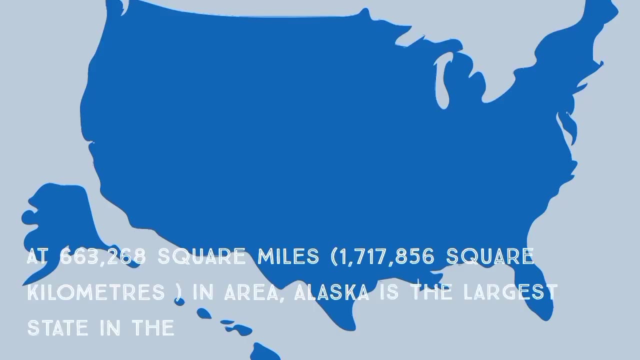 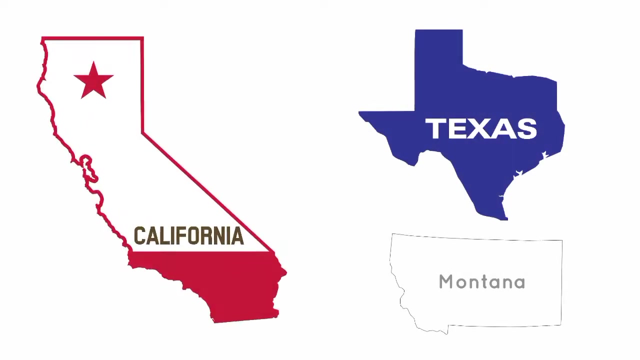 At 663,268 square miles in area, Alaska is by far the largest state in the United States and is more than twice the size of the second largest US state, Texas. In fact, if you combine the area of Texas, California and Montana, it would still be less than the size of Alaska. 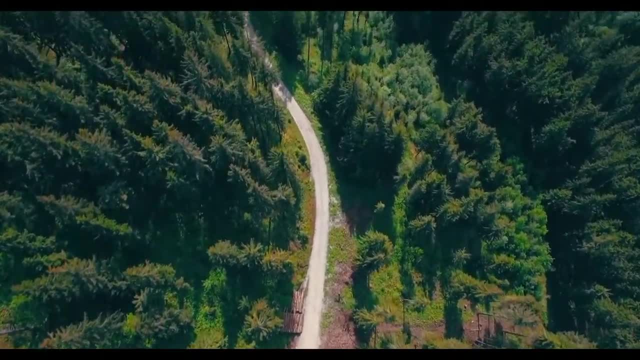 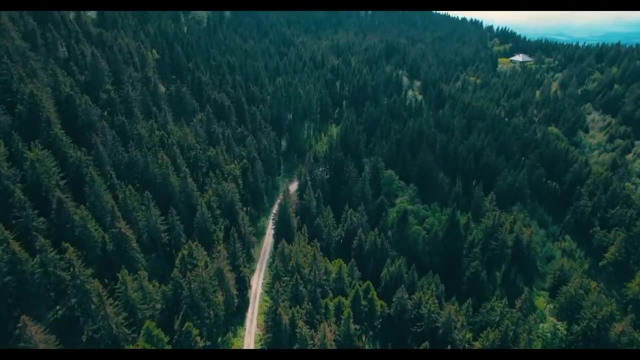 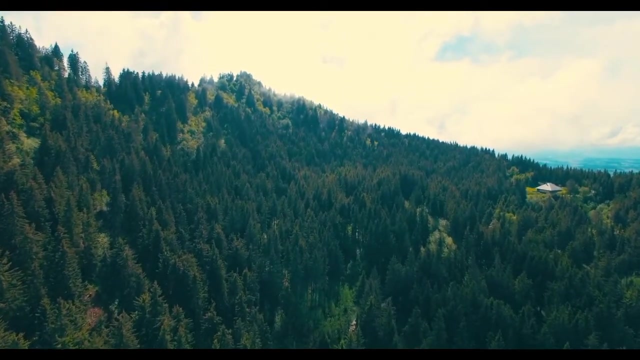 Alaska is big. what if it was a country rather than a state, Considering that Alaska is the seventh largest subnational division in the world and if it was an independent nation, would be the 16th largest country in the world? Alaska is as big as England, France, Italy and Spain. 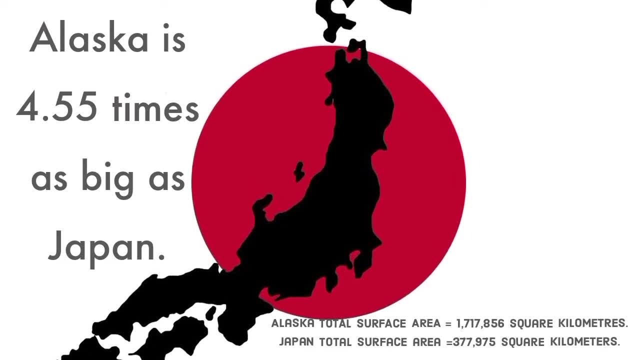 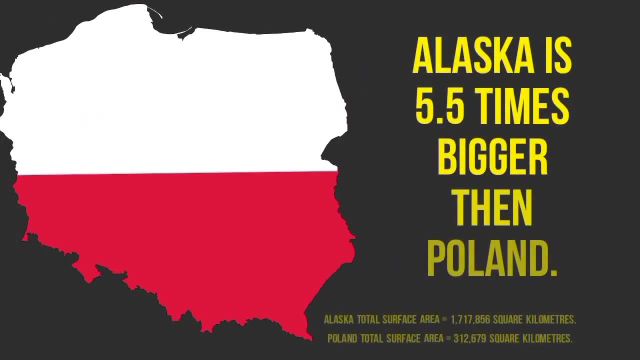 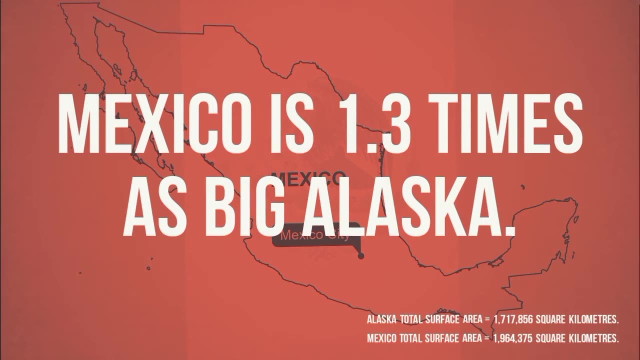 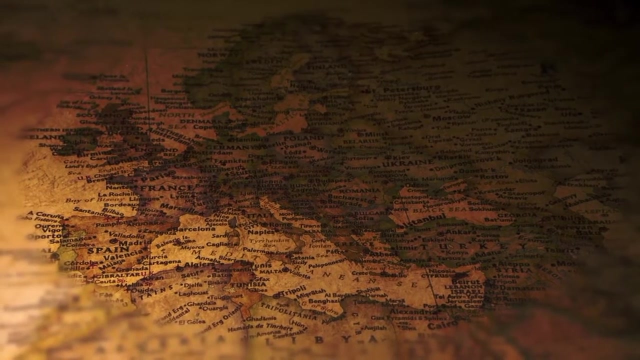 combined, Alaska is 4.55 times as big as Japan, 4 times bigger than Sweden, 5.5 times bigger than Poland, while Mexico is 1.3 times as big as Alaska And Russia is nearly 10 times as big as Alaska, While Europe is 5.93 times as big as Alaska. 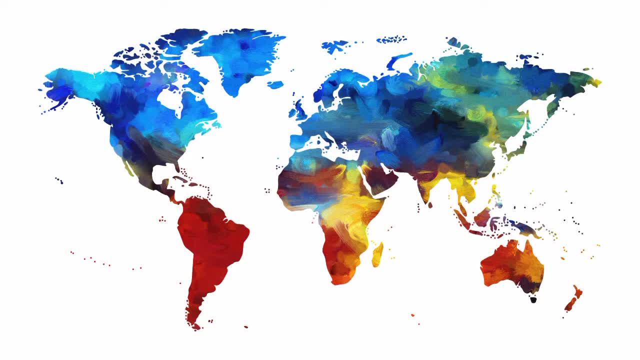 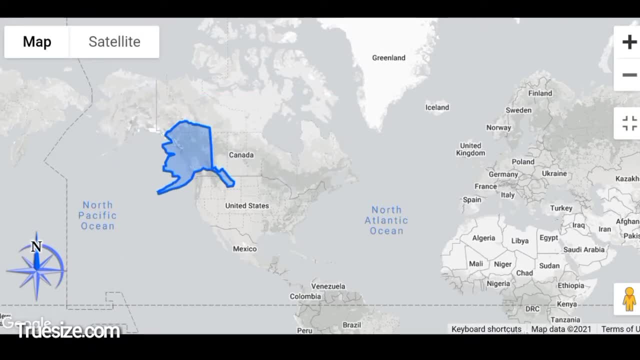 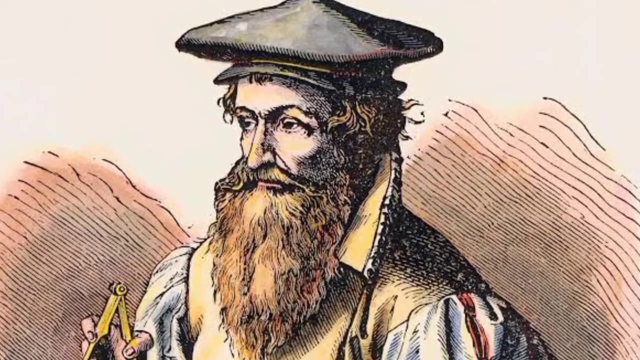 When you look at world maps, Alaska will look so much big in size. well, it's not true. Its size is greatly exaggerated. this happens because most of the world still uses the old Mercator projection type maps. The Mercator projection was developed by Gerardus Mercator in 1569.. The Mercator 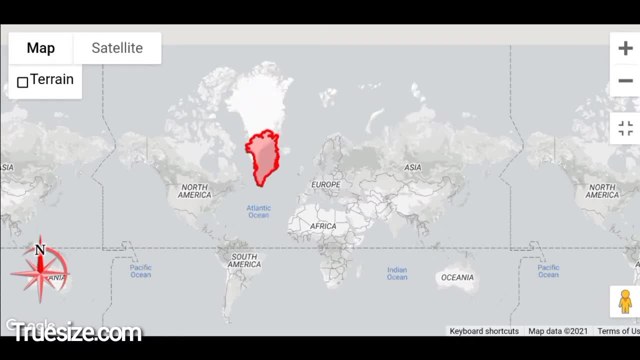 projection drastically distorts the size and shape of objects approaching the poles. Places closer to the poles looks much bigger, while places closer to the equator look small. That's why Greenland looks so much big in size on a world map, On a typical Mercator. 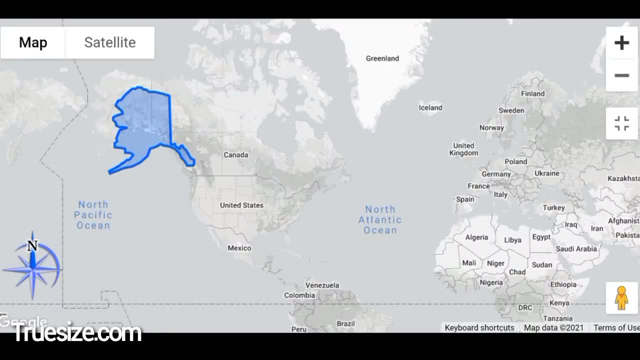 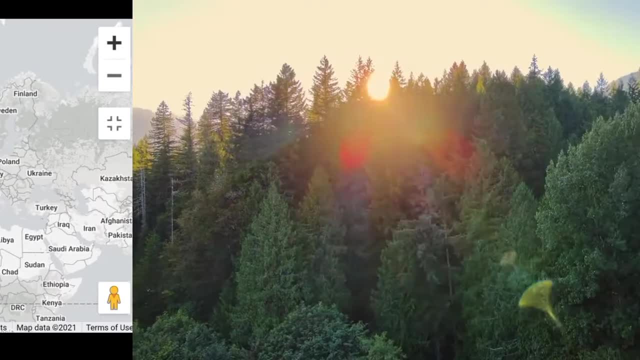 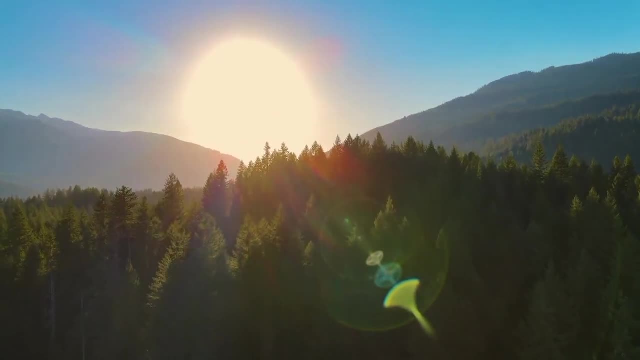 map, Alaska appears to be more than half the size of the lower 48 US states, when in reality the continental US is 4.7 times as large. In 1865, Greenland purchased Alaska from Russia in 1867 for $7,200,000 dollars- about two cents. 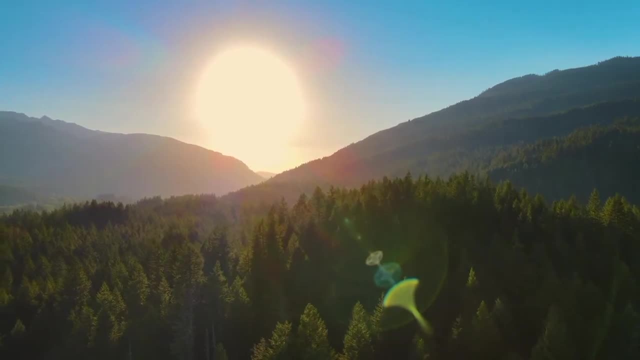 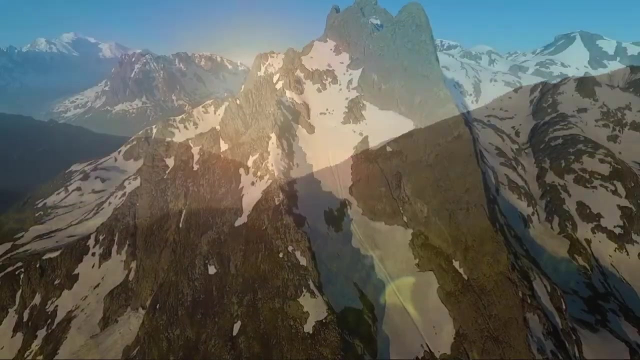 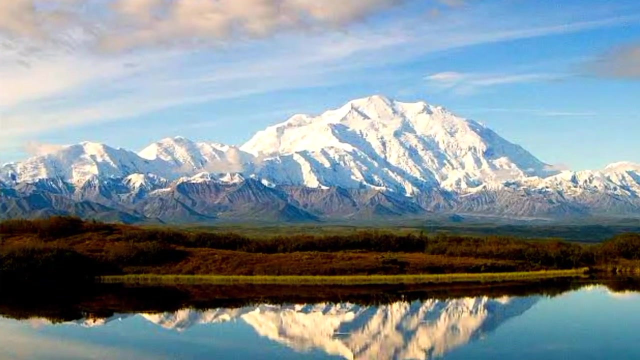 an acre and made it the Union's 49th state on January 3, 1959.. At their closest points, Alaska is approximately 55 miles from Russia. Alaska has 17 of the 20 highest mountain peaks in the United States. Denali is the highest, at 20,320 feet above sea level. There are